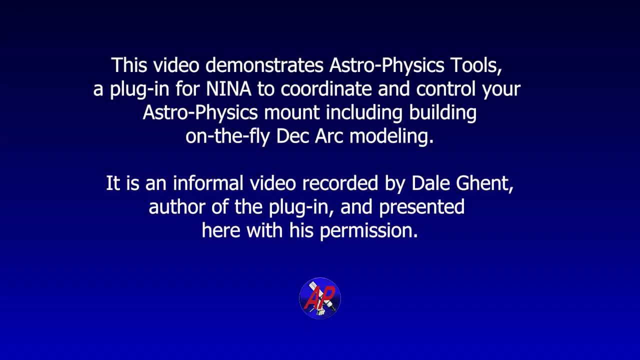 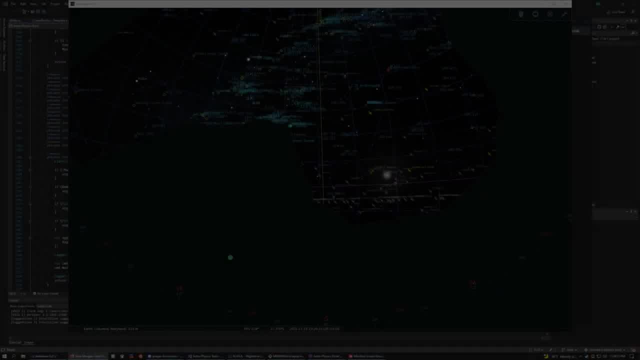 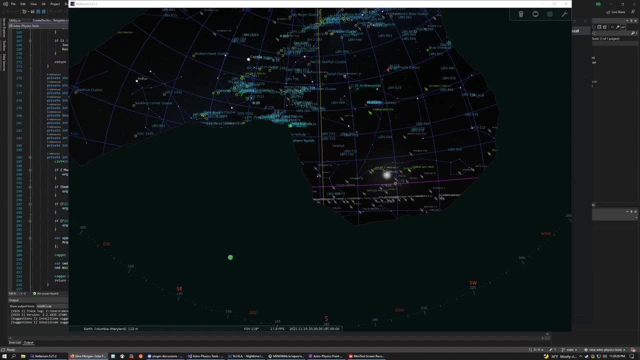 Hey everyone. this is just a quick update on the progress I'm making with the create DECARC model instruction for NINA's Advanced Sequencer. It's part of the plugin called Utilities for Astrophysics Mounts. I'm renaming that plugin by the way it's going to be called. 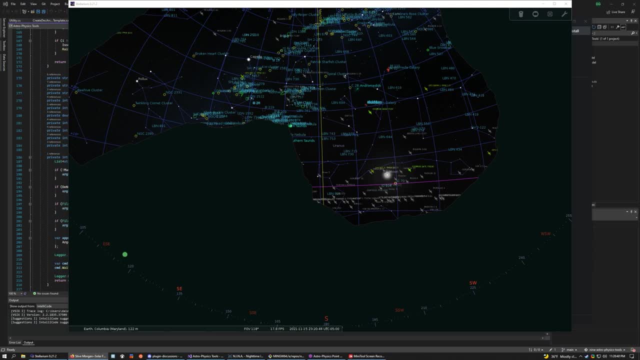 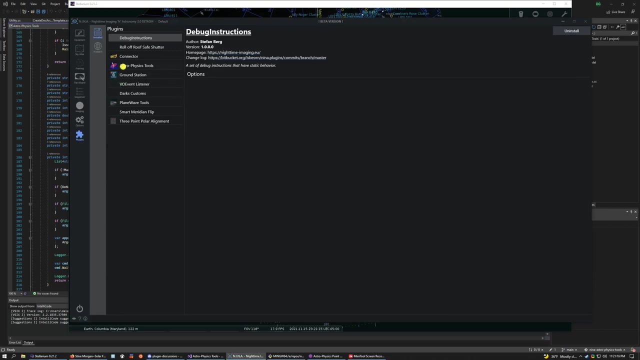 Astrophysics Tools after the next major release, And what we're going to do is just step through how the instruction works in conjunction with Astrophysics Point Modeler, APPM, and how the general configuration regime and the ways you would go about utilizing it within your sequences. For those who aren't familiar with what a DECARC model is, 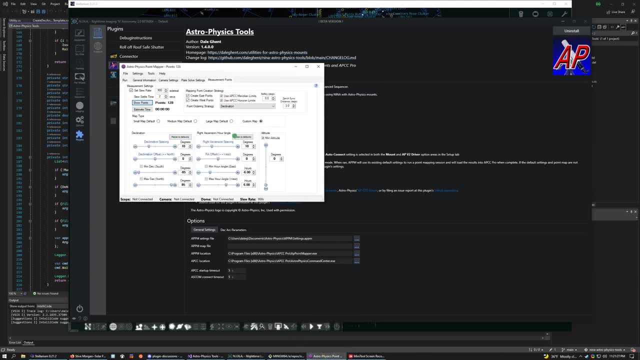 let me pull up Astrophysics Point Modeler here with the default set down here in the declination and right ascension. The point mapping of course lets you map deviations in the expected or from the expected. in the sky. Air has refractive qualities. There's various. 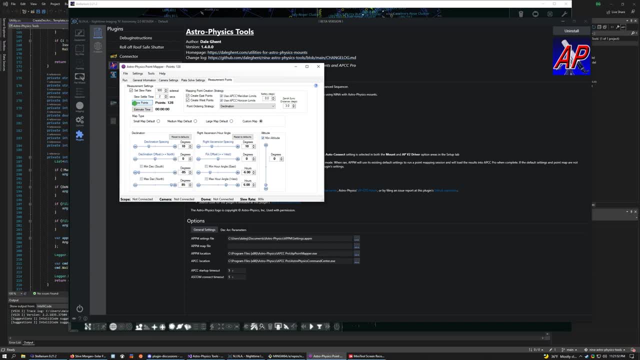 densities of air floating around up there from you know, bubbles of cold air and hot air and stuff like that that refract light ever so slightly differently than surrounding air. And there's also things like flexure, mechanical flexure on air mounts and stuff like that. 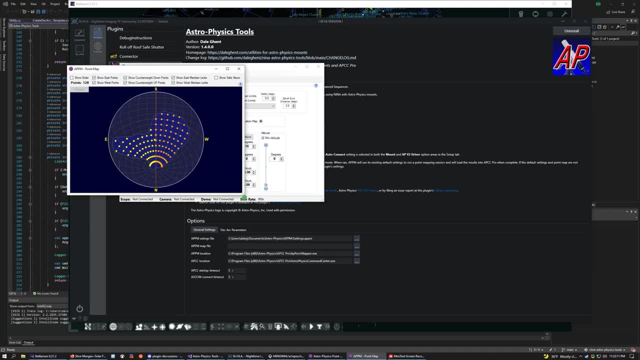 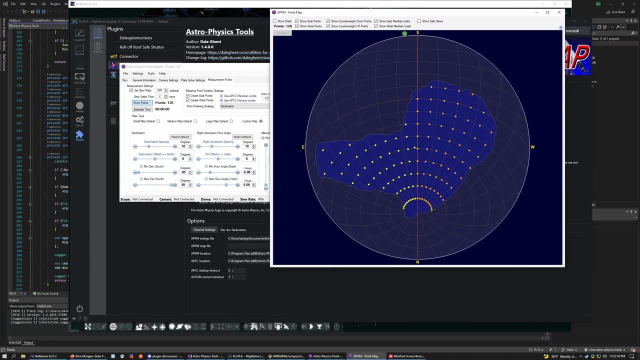 And the sky modeling is is meant to basically survey that and model it so that the APCC can then adjust the rate of which the mount tracks on the fly in accordance to the model, And so the mount might speed up a little bit, it might slow down a little bit, depending on what part of the sky it's in. 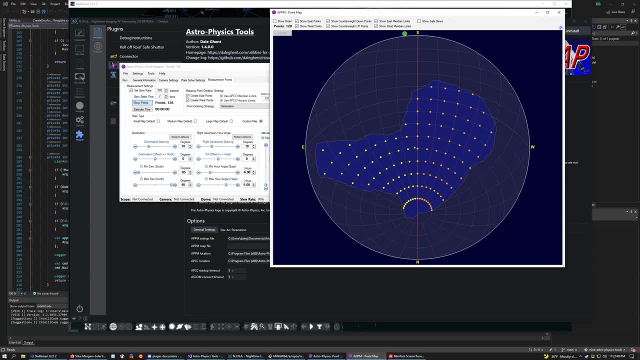 based on what the model says, And it's one way to get very accurate guiding and it's absolutely key to getting doing unguided exposures. So typically, the sky, the entire sky, has always been modeled, And so what we see here is an example of this. You see, my local horizon here is overlaid, And if we remove, 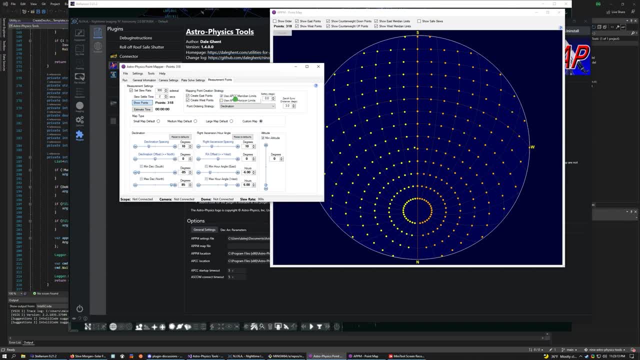 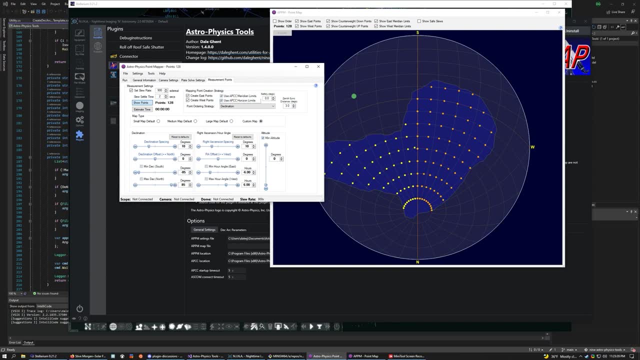 that, then you can see that it's overlaid. And if we remove that, then you can see that it's overlaid. see, the whole hemisphere would look like, But the reality says I have trees and houses, and so this is the slice of sky that I see. Therefore, it's the slice of sky that we should. 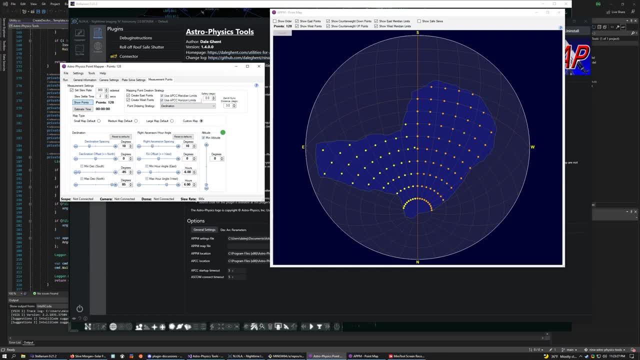 really model. So that's the first kind of takeaway here is: if you don't use horizon limits within APCC and thus in APPM, then you're missing out. You should really put those in so you don't do more work. But that's the first kind of takeaway. if you don't have horizon limits within the APCC and thus in APPMSam, Spitz is missing out, You should put Wildr은utog- The reality, that's the32nd triangle- in there, and sky, sky is missing, And you should really put those in So you don't do more work. 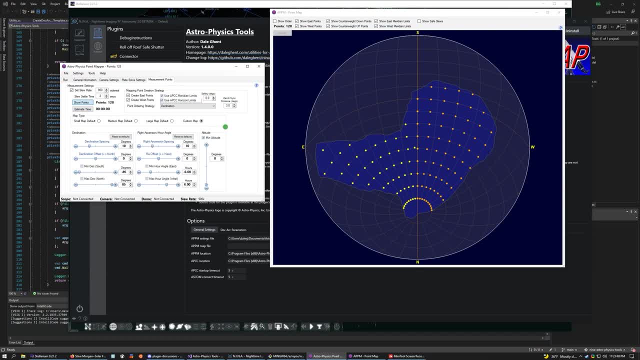 terior concerns 明 than you have to. so, but here's a basic example of an all-sky model, and it literally is the whole sky. the APPM will take images at each one of these points and feed that into the model, and and there you go. but you know, as 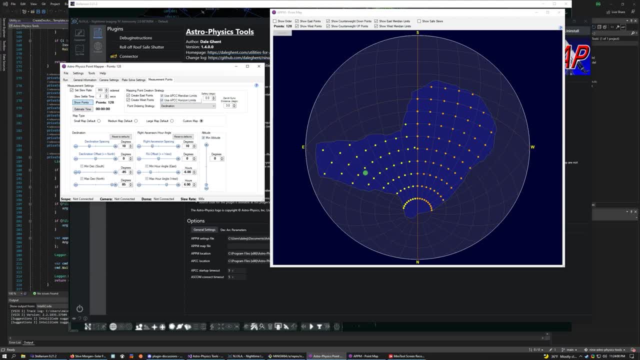 astrophotographers were usually concerned with one, maybe two targets, rarely more than that on a given night. so this whole sky model. if we were to model this whole sky, or just imaging something you know around 60 degrees declination, then all this other time spent here modeling these parts of the 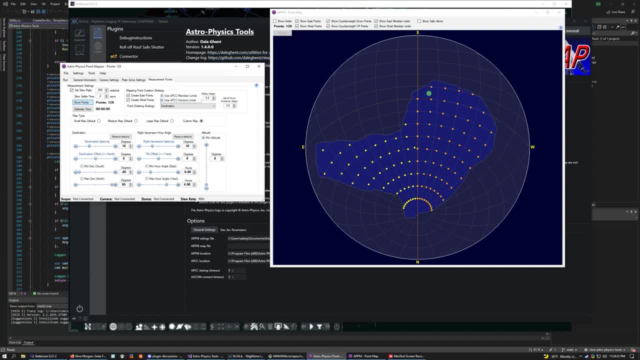 sky that will never look at this time wasted. so I mean, what if we could take all that time and just model the area of sky that we're gonna be imaging? and that's what a deck arc model does. it just models the area of the sky that you'll be imaging. 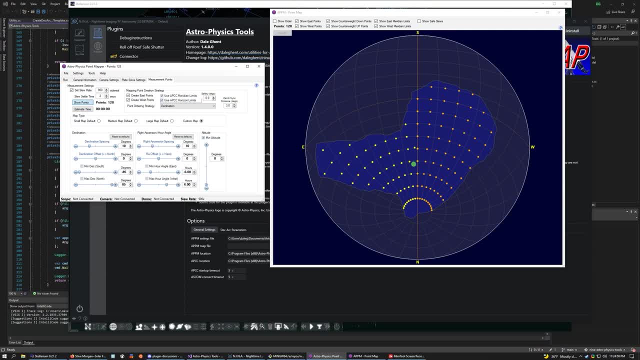 in. so, as you can imagine, where, as an all-sky model is kind of like the shotgun approach, deck arc models are the surgical approach. but to be surgical you need to have kind of a relationship, a working relationship between a PPM and the sequencer, and so that's where my plug-in comes in and this deck. 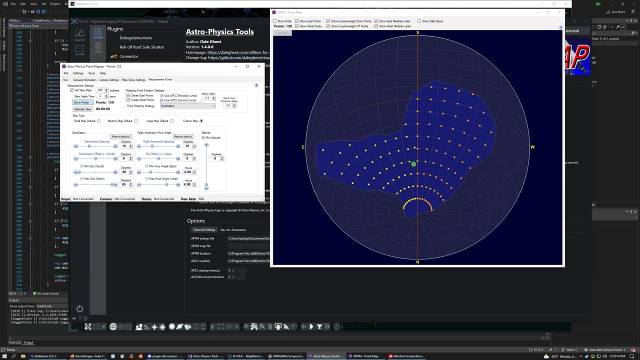 arc model creation instruction for for Nina. so basically what it'll, what the instruction will do is when you start imaging a target and it'll say, oh hi, you have a target. it's RA in deck is this? I'll generate these parameters for APPM and send APPM off to create a model that's suitable for the target, based on its RA and 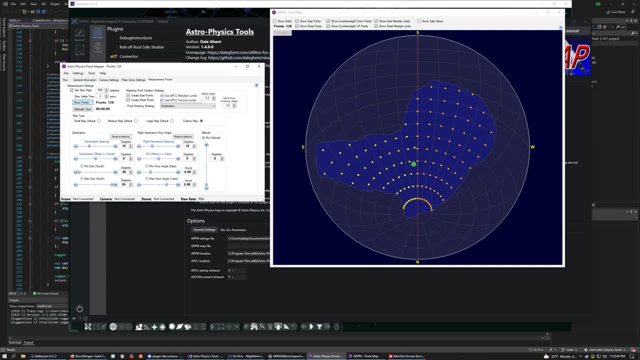 declination And we'll load it into APCC and then commence with imaging the target with that model active. So it's on-the-fly model creation and completely automated. So you don't need to do anything manual to facilitate this process. It's basically you press, go in NINA and 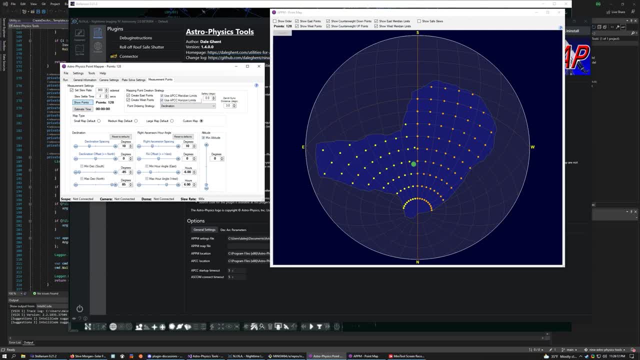 when it hits the create APPM, the create DECARC model instruction, it makes it, And then the rest of the sequence goes on. whatever you're doing- imaging a narrowband or whatever- So let's start. Take a look at what a DECARC model might look like here in APCC, And so I'm just going to roughly. 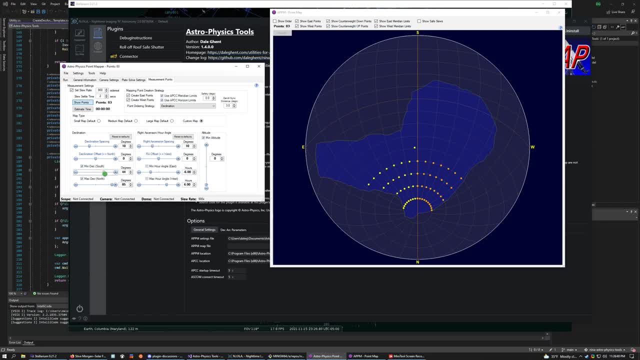 approximate one. So you know, say we're imaging something around 60 degrees, so we'll cut down there. there, Let me decrease the spacing and decrease Yeah, So. yeah. So say we're imaging something that's in this area of the sky and we're going to image it towards the Western Horizon. Well, 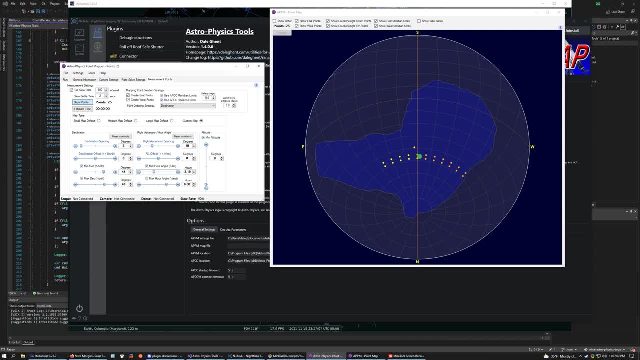 this is what the DECARC model would roughly look like Is. you know the target would be in between these two arcs of declination. that are models And you know we're going to image it from this point westward. So, and by default, this plugin, this plugin will start. 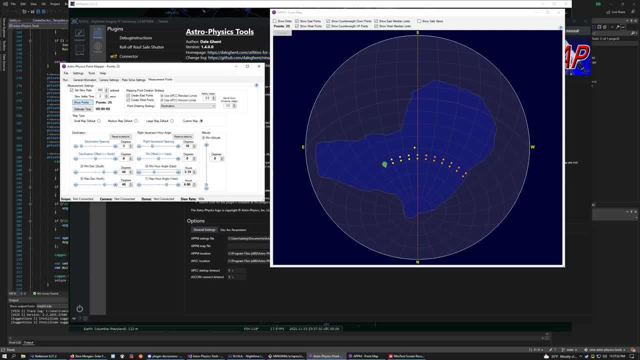 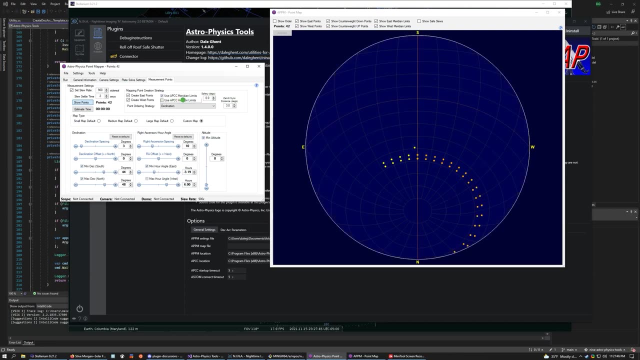 image start the model creation. at the current hour angle of the target, the western extent of the arc is going to be whatever your horizon is, and that's why it's important to have these horizon limits in apcc. um, yeah, yeah, you could ask the question. well, you know if, um, you know if i'm, if i'm going to. 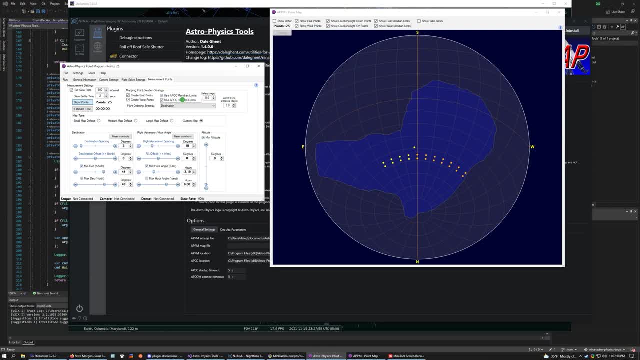 image the, if nina's going to image the target to their horizon, anyway, why? why, you know? why can't nina just calculate when that would be? and well, that's true, but there's other things that could end your um, these other conditions that could end your imaging, and sometimes these conditions, 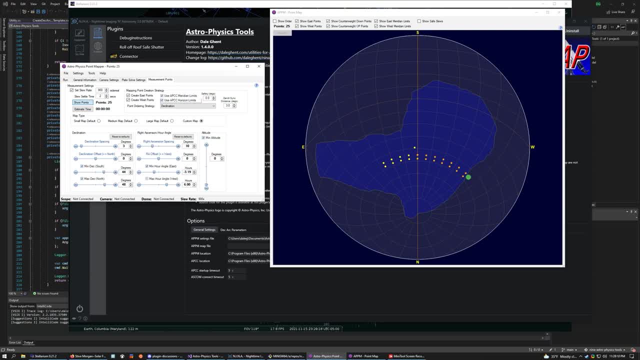 aren't predictable. so, uh, you know, while we know where we're going to start imaging the target, we don't really know when we're going to image this target, um, and so that's why we say, well, just image, just make a model to the farthest extent. 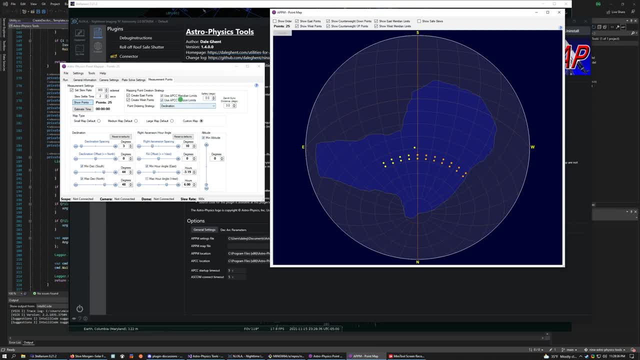 that you can, which would be either your local horizon, if you're using apc horizon limits, or zero degrees on the horizon, which you don't want to do, unless you live in texas and you have a zero degree view of the sky all around. plus, most people don't tend to image below 20 degrees or something like that. anyway, because of all the 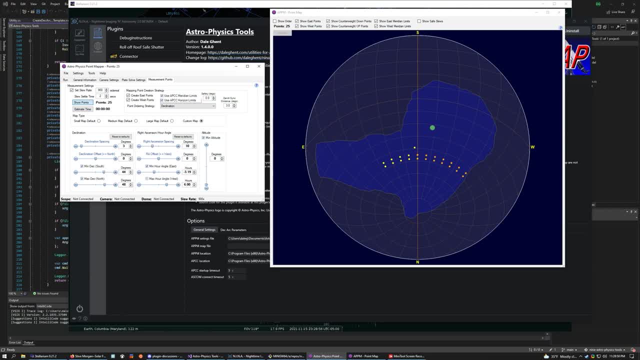 muck and murk in the atmosphere. so, um, again, another shout out for using horizon limits in apcc anyway. so what the instruction will do is create a, an appropriate um set of parameters for appm to make this kind of model, and we'll go over those now in nina. 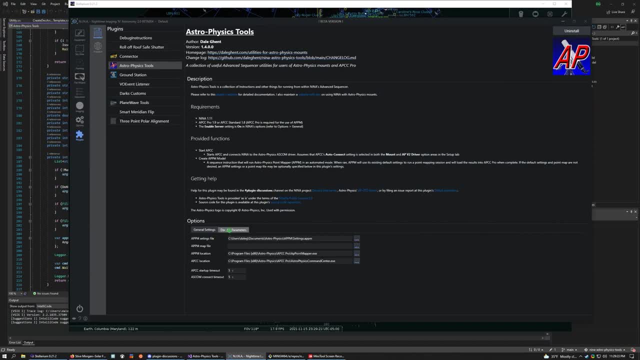 so, uh, first thing you might notice about the plugin is that the options area is now tabbed and deck arc parameters has its own tab and the knobs are, i think, kind of straightforward. we specify the quantity that we want to um, that we want to image and uh, uh, you know, generally around 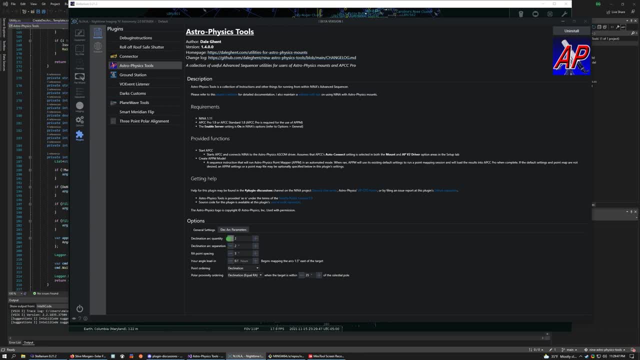 two or three arcs? um, if it's two arcs, the target will be somewhat centered in between the two arcs. if it's three arcs, then there will be a central arc that goes over or is very close to the the target, and then one arc on either side, and all these arcs are separated by 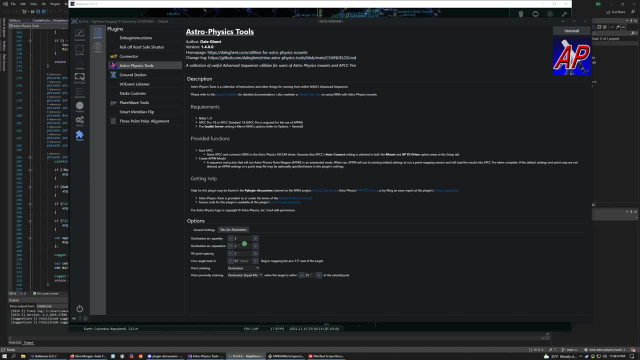 the specified declination, arc separation, so all the arcs can be separated by two degrees. so, uh, you'll have the central arc and then, uh, a northerly and a southerly arc, two degrees on either side of it, two degrees away on either side of it. um, all right, point spacing, uh, dictates the. 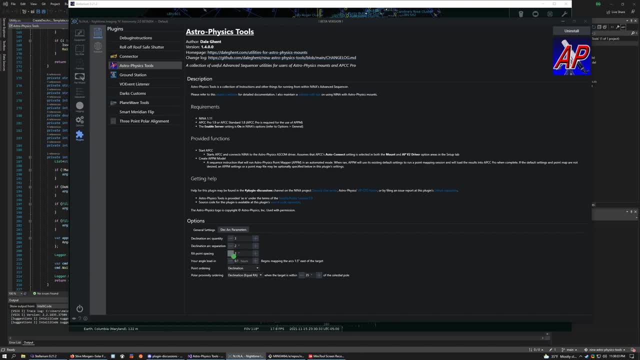 basically the, the density of points along the right ascension. so this says we're making a point every three degrees. um, you know, you can make that less dense by saying a point every five degrees, or more dense, a point every two degrees. it's, it's up to you. of course, the more points you. 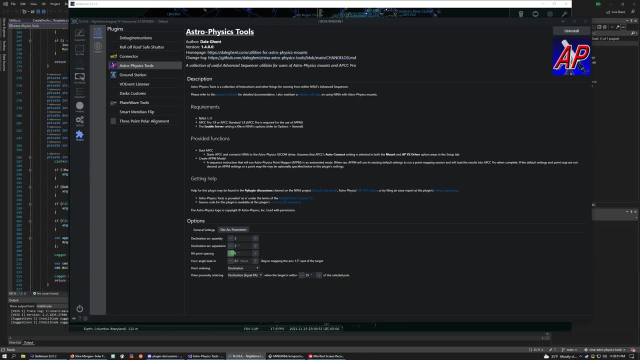 ask for the longer the model will take to create um, and so those are the three main knobs there to adjust things with our angle. lead in um. our angle is uh, um, this is so by default. nina will will start creating the arcs where the um target is currently in the sky and um, and so what you can do here is say: well, i want to. 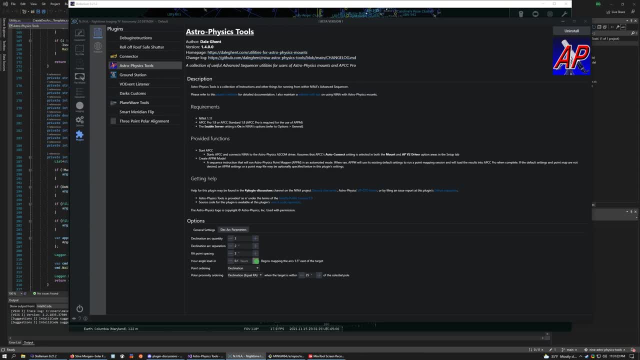 uh, i want to start creating the arcs. um, uh, you know, a little further east, for whatever reason. um, so you can specify that here, an hour angle lead in so one, you know, one tenth of an hour is one and a half degrees further east than the target's current position. so i mean, if you want to, you can, you can have it. 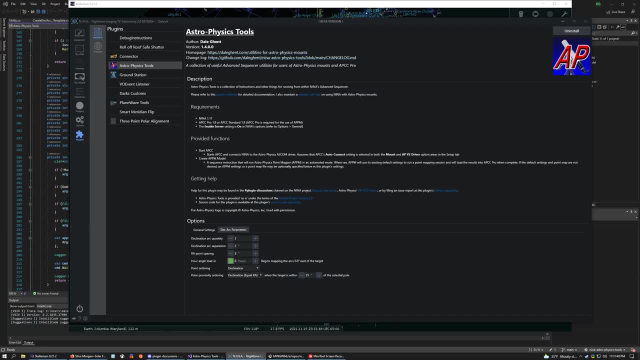 do a full hour, if you want. remember, one hour is 15 degrees of sky, so that's, that's the divisor there. um point ordering: this is detailed in the astrophysics point modeler, or appm uh, documentation. this governs how, um how, the how the points are, um spread. 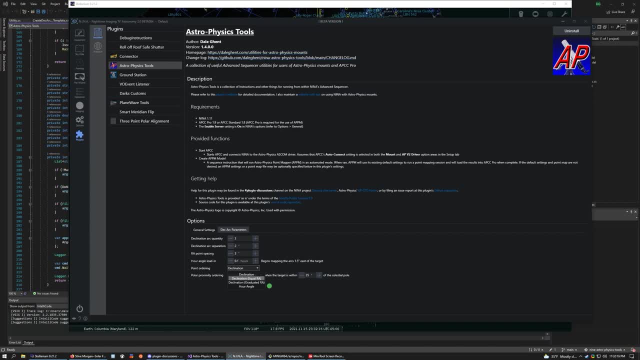 and how they're, uh, in what order they're imaged in, and this may not have much um importance when you're imaging um farther away from the pole, more towards the celestial equator. it does have more bearing, though, and more importance when you, when you, get closer to. 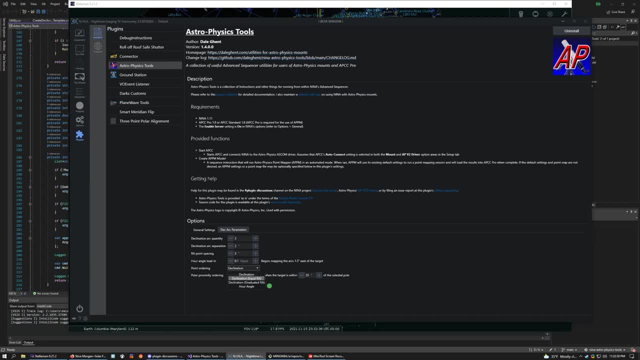 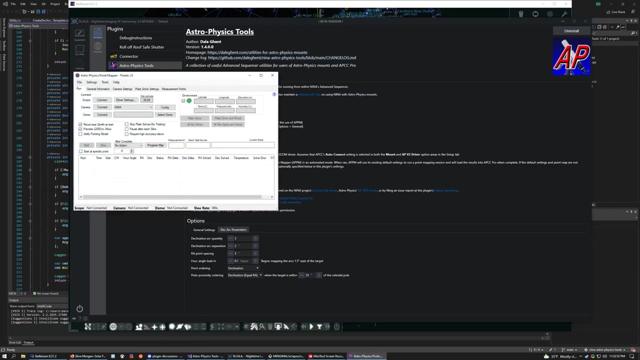 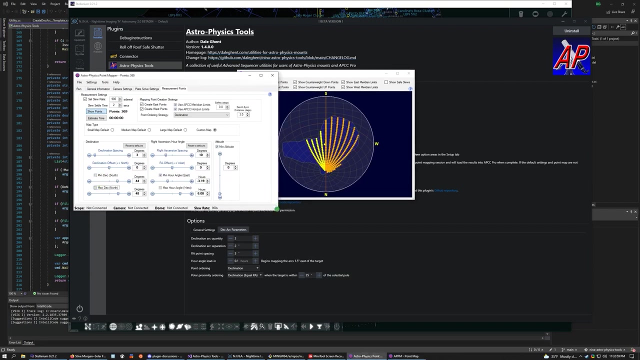 imaging: uh to the pole, to the to to the celestial poles and um, uh, if we, if we go back to our astrophysics point modeler, uh, our point mapper, uh model over here and let's expand this back out, we can see, with the declination point ordering strategy, that 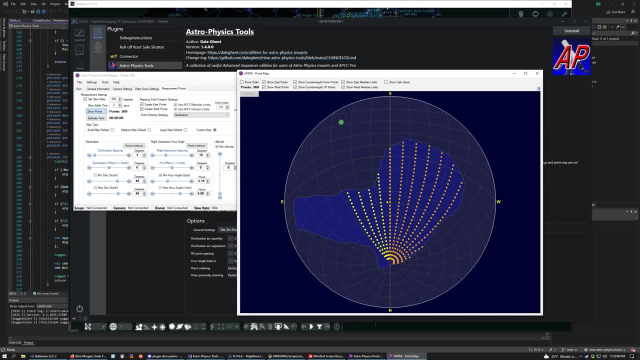 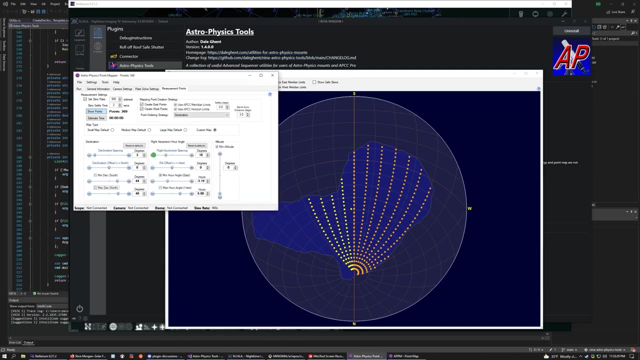 things are kind of sane around the, the middle. uh, you know, farther away from the celestial pole. once you get towards the celestial pole that's quite some density there and, um, especially if you, if you reduce the ra spacing, that gets a little more wild down here by the pole. 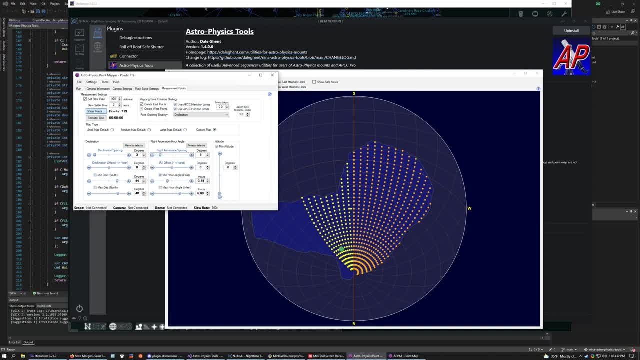 and um, it vastly increases the um, the um, the number of points you have to model. so if you're imaging down like close to the pole, that's an awful lot of points to to to deal with. so, um, these other options- here in point ordering strategy- can alter that behavior. so if we 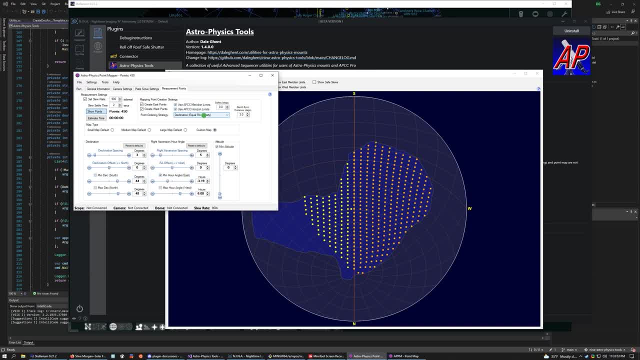 switch that to equal ra, density, um. the density of the um of the points as you get closer to the celestial pole is adjusted so that you don't get that kind of harried mess. the math is explained in the astro in the appm document. graduated is another form, so you can see the difference here between the two. 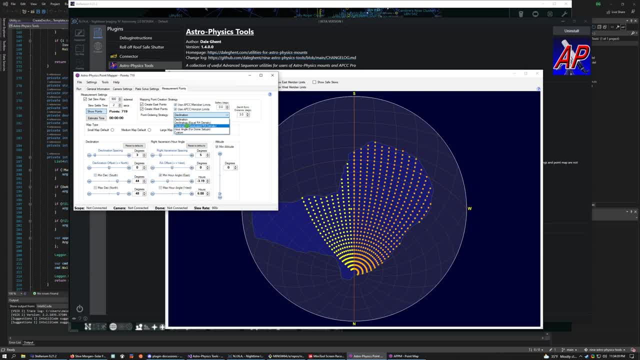 um, it's kind of like an in-between of equal ra density and and just basic declination and, of course, um ordering by our angle is is another optimization that's aimed at domed setups. um, so, normally, what would what? what appm would do is, uh, is image, image these points by declination. so it goes, this, this declination, they go to the. 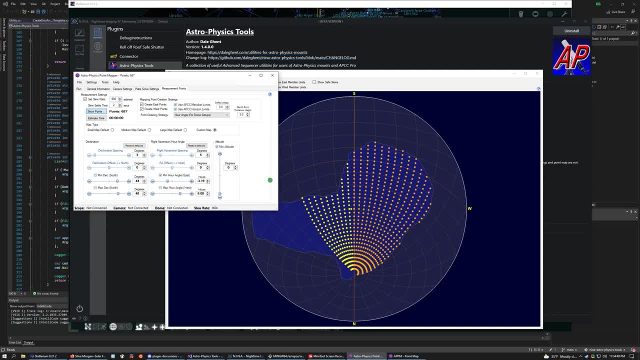 next row. this is it east to west, and this is east to west, and it's going to go north to south. so if we go to the left and we go to the right, we can image those dots. our angle ordering strategy changes that so that it goes up by our angle. so instead of going east to 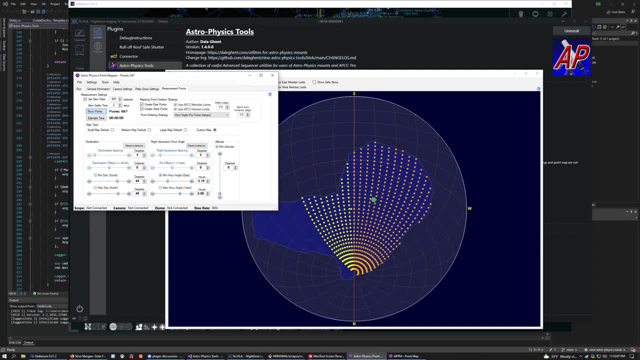 west. it's going north to south, and and so the goal of this is to um minimize dome rotation movements, and how much the dome rotates will depend on its, on your dome geometry, um, your the field of view of your optics, and so on and so forth, but um, uh, that's kind of a. 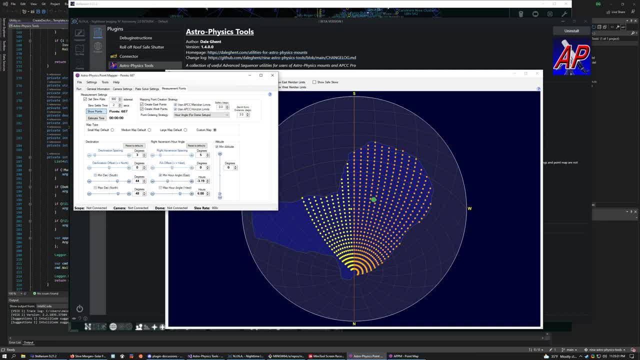 situational thing it's having it do our angle is probably more important for these, uh, these middle latitudes here, um, in the sky, um, then it probably will be down here by the pole, down here by the pole. the points are so dense and close together that you might want to do, you know, equal ra. 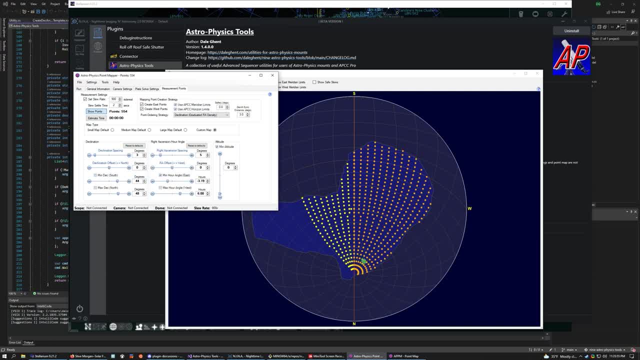 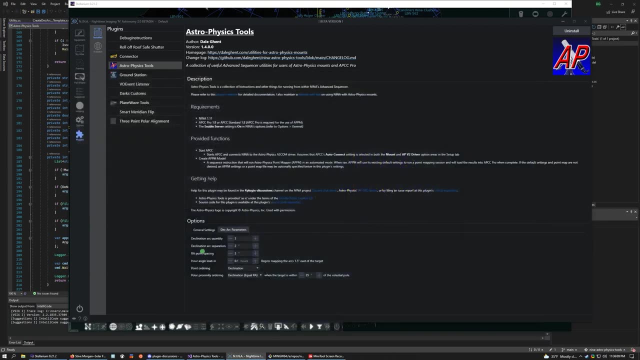 density instead, or graduated uh, instead you might get some more dome movements. but um, again, it's your call, um, you kind of have to pick out what works best for you there anyway. so that's what that setting is, and so it's a two-step setting. so, like i said, um things get. 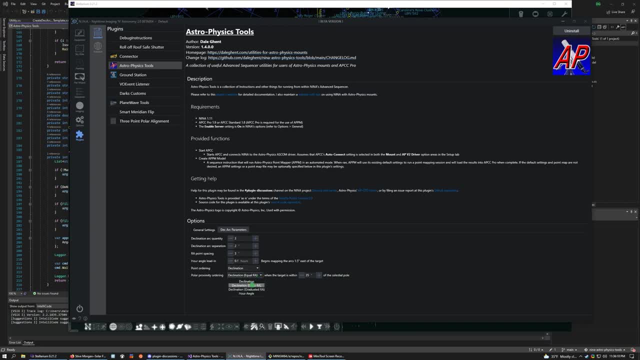 crazier by the poles so you can pick a different um or ordering uh based on the proximity to the pole. so this says we'll do equal ra when we're within 35 degrees of the celestial pole and uh and so the the ordering can be changed on uh automatically if the target's within that zone. 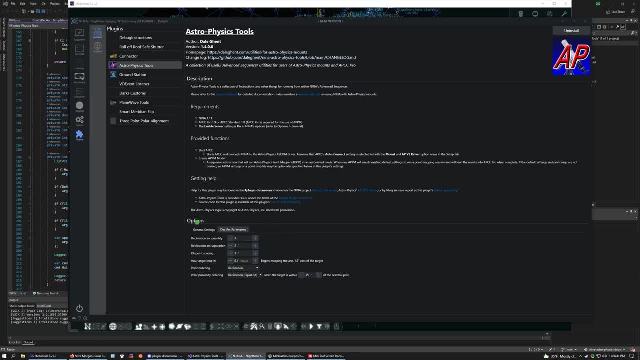 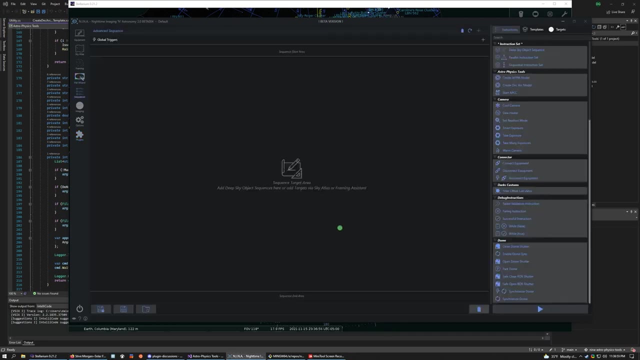 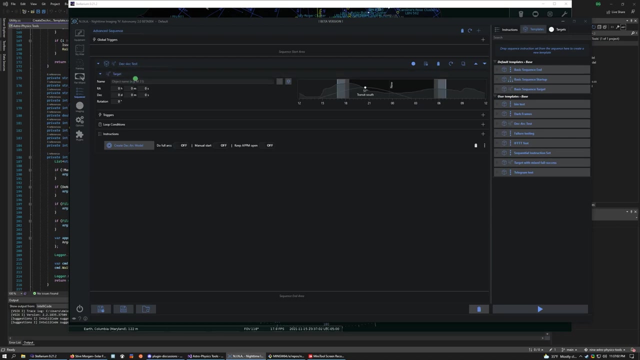 um. so that's basically the parameters. so, and in practice, this will uh um, this will uh um work out like this. so, uh, we'll go to the sequencer. we've got a blank slate here and, uh, i've got a template here called dakar test, and dakar test is basically just a dso container. 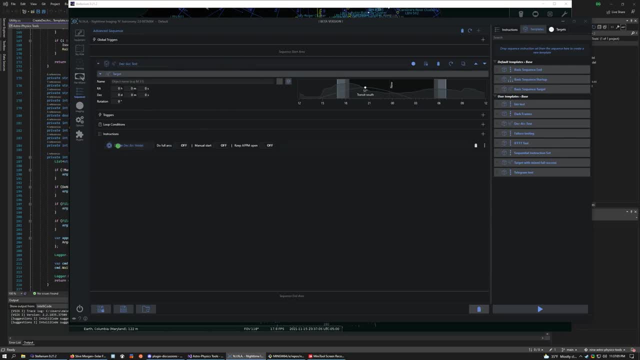 with just to create deck arc model um instruction in it. and, by the way, there's three runtime options for this. there's do full arcs in this case, and then there's the do full arcs in this case, and then there's the do full arcs in this case, and then there's the do full arcs in this case, and then 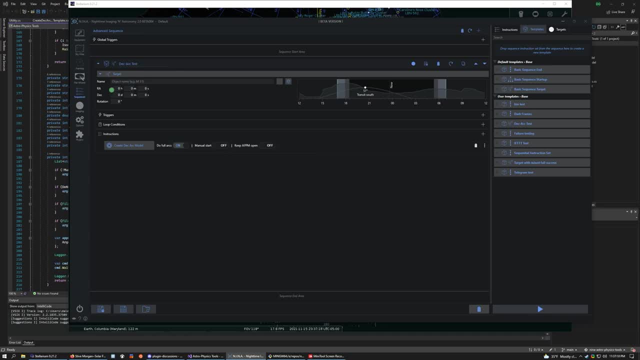 basically says: i'm going to do a full. i want to ignore the- uh, the current hour angle of the target. i want to do a full horizon, horizon arc modeling of the target's declination. um, you know, default is off, obviously for that manual start. that means don't start. 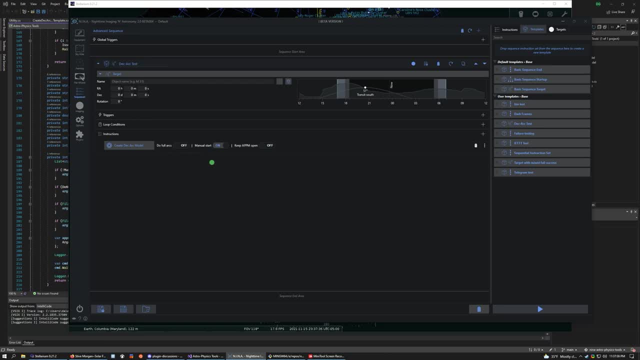 appm in automatic modes. so this will just launch a ppm with the parameters loaded in it. you will still need to manually connect the camera and telescope and dome and then start the model to keep it. you know to go and then quit a ppm. so it's, it's full. 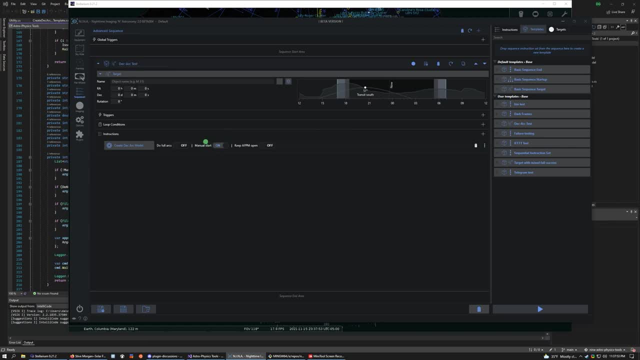 manual mode. the only thing it does for you is start a ppm and load the parameters in and then, if you're running an automatic mode, you can create, you can keep a ppm open at the end and you know this kind of lets you review the model. before the rest, you know the rest of the sequence progresses. so if you wanted to, 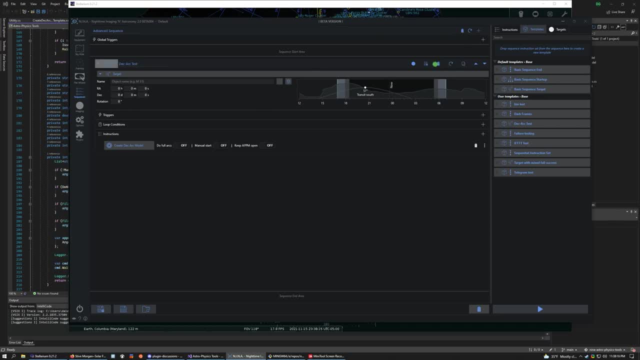 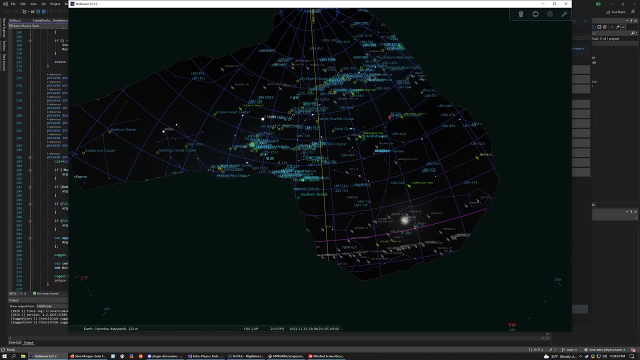 do that. you can do that there. so what we're gonna do is we're just gonna pluck a target out of stellarium here. we're gonna pick one yellow line. here is a meridian. east is on the left, west is on the right. we're looking south here and 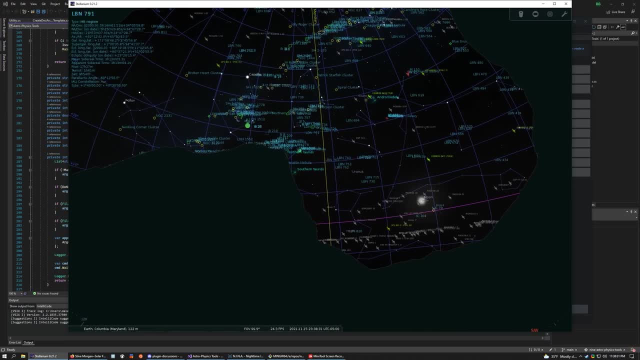 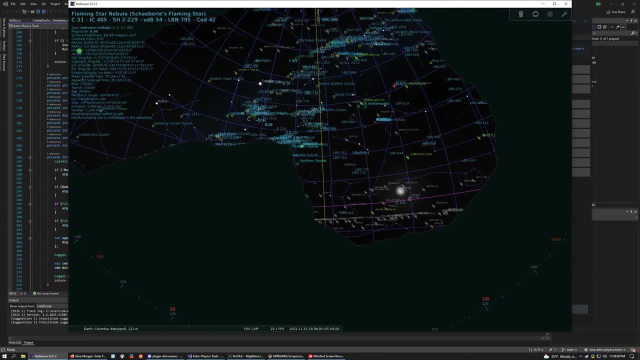 so I'll pick. yeah, what about? what about the flaming star nebula? there seems good, all right. according to stellarium, it has an hour angle of, and this is European. Western, our angle is negative 12 to positive 12. European, our angle 0 to 24. 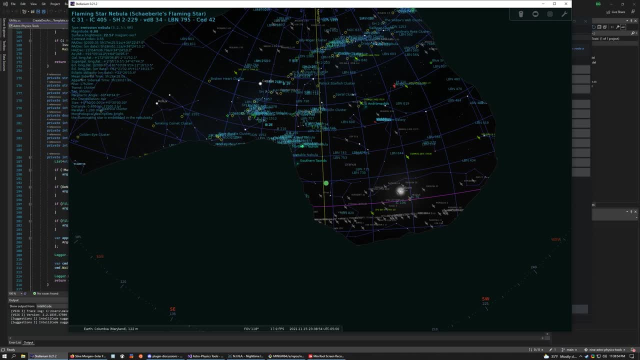 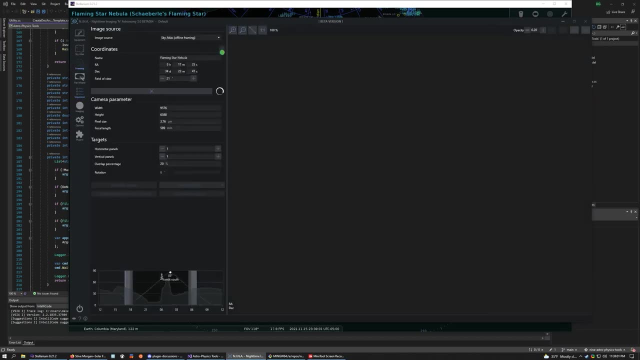 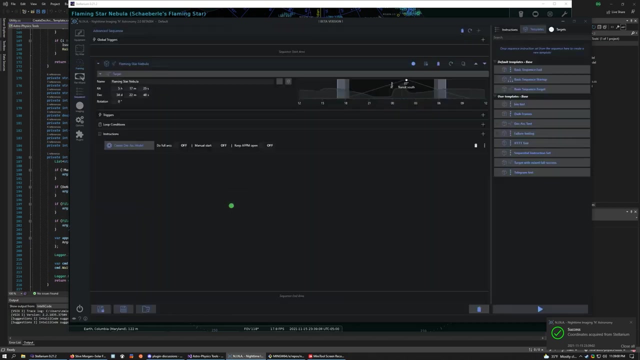 so we're at 24 hours zero being the meridian. so we're gonna go over to framing wizard pulled out of Stellarium and then we're just gonna make a sequence out of it using that DeckArq test template. here it is loaded in. so 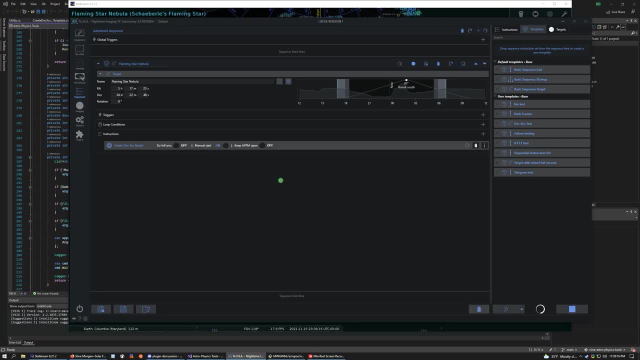 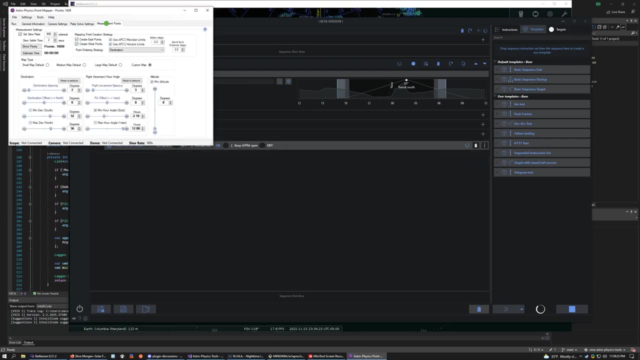 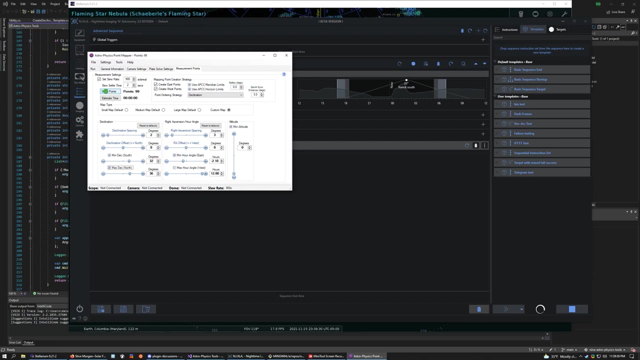 So we'll turn on manual start here and hit play. So the instructions running, it's generating the parameters and it started a PPM And that was supposed to be on. but so what we're going to do is we're going to show points. 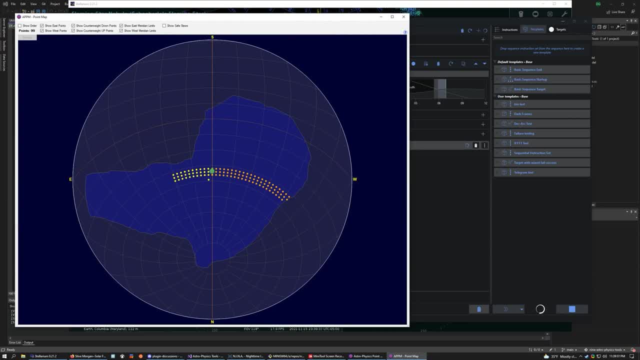 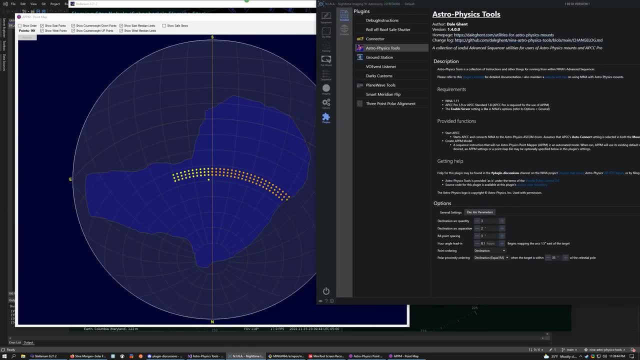 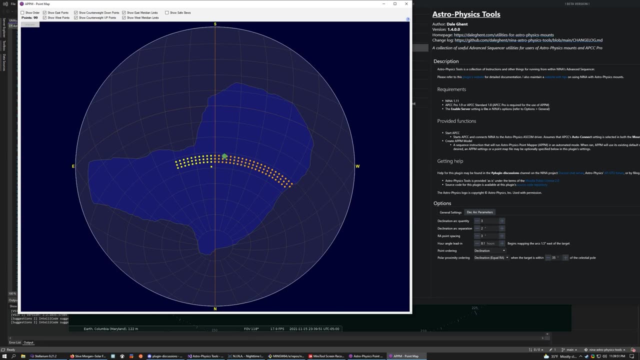 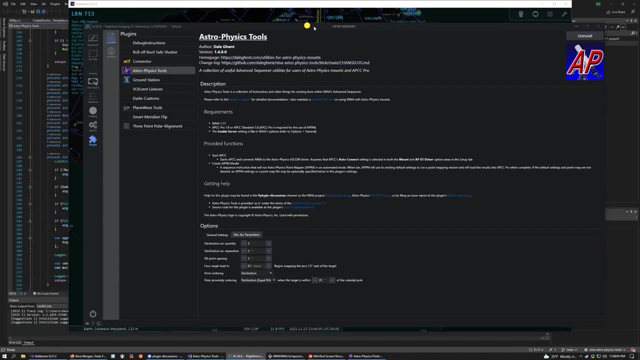 here, And so we have our three declination arcs in accordance with our parameters: Three arcs two degrees apart and RAA every three degrees along those arcs, And so that's what will be modeled. It's that straightforward, So we can go in and pick. 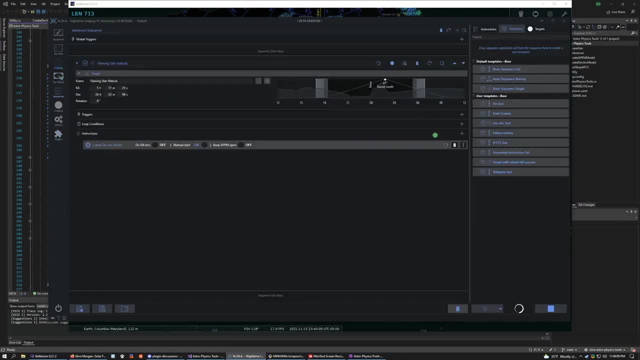 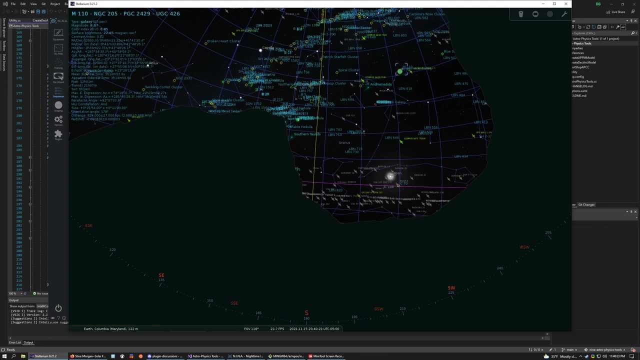 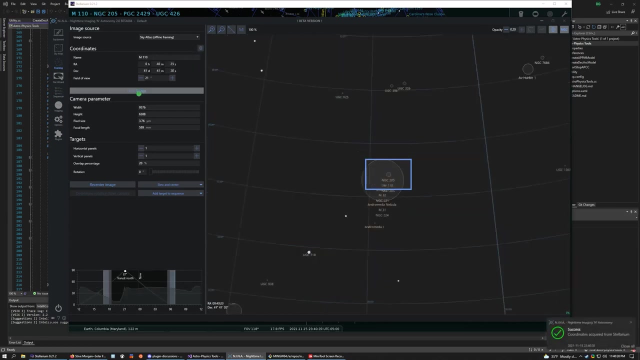 Okay, Okay, Let's see here: Well, let's first shut that down, clear that, and we can pick another target. And let's say we're just going to do a start, a late start, on Andromeda here And pull that in and create our deck arc template and go. 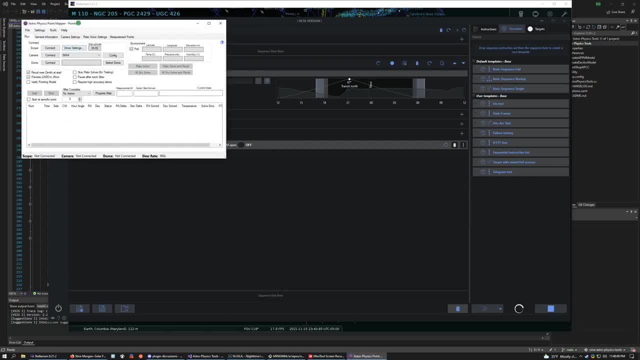 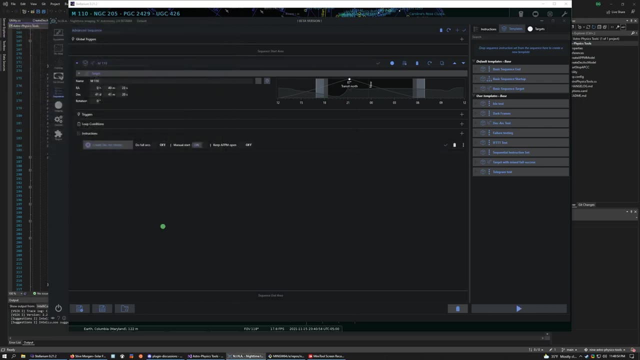 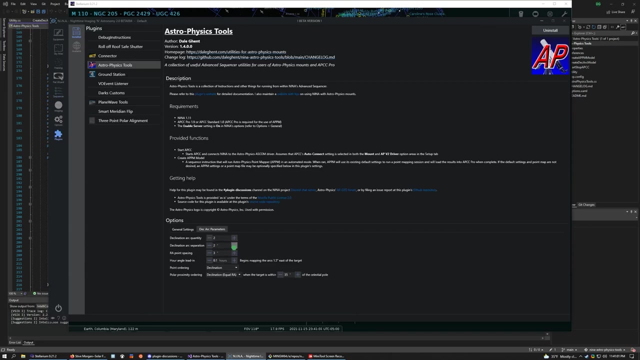 Okay, There it is, 25 points. Take a little over six minutes to do. We'll look at it here. There we go. What we can do is reset this progress, go over here to our plugin settings and say: I want to do two arcs five degrees apart, with RAA spacing every 25 degrees. 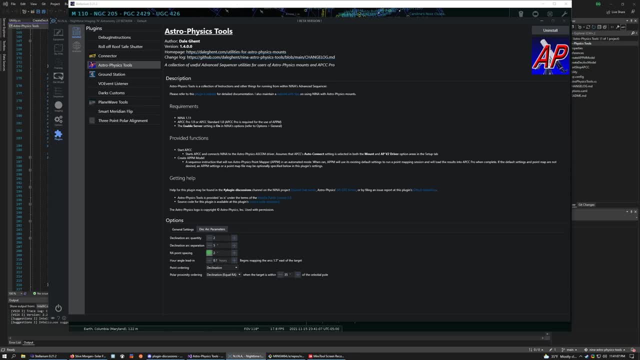 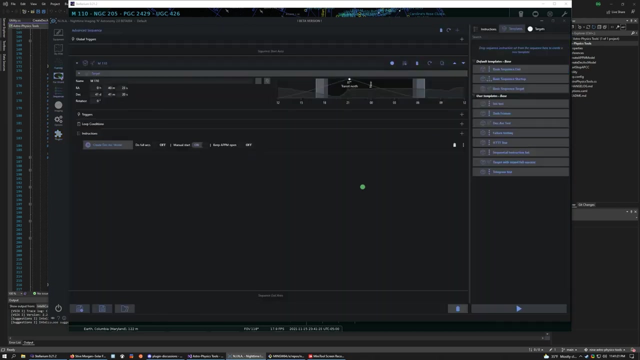 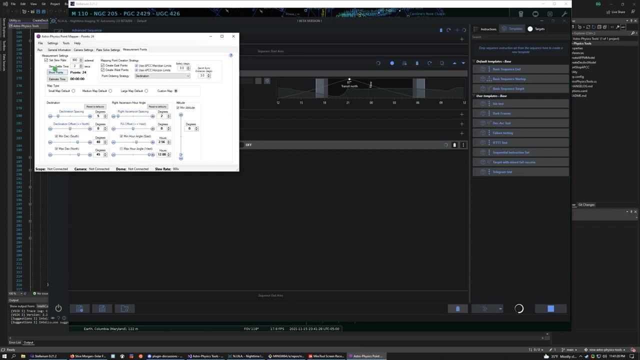 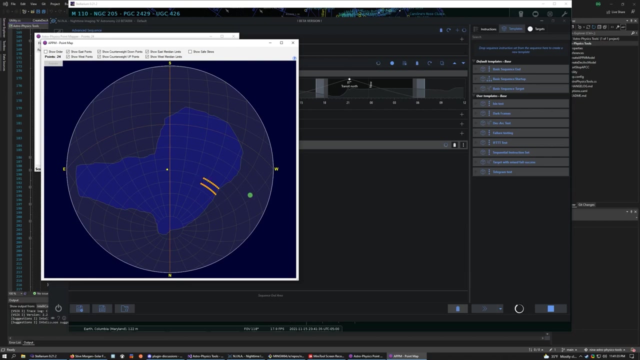 Okay, That's what we're going to do. There we go every two degrees and I want, I want to bump that back by four and a half degrees. so do that. go back to the sequencer, run our model again, take a look at our points. and we've got our we've, we've got our parameters reflected. 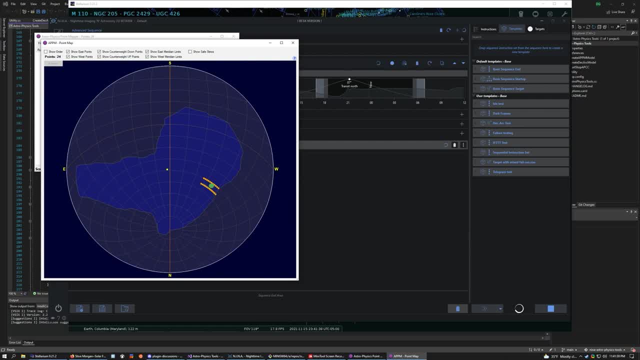 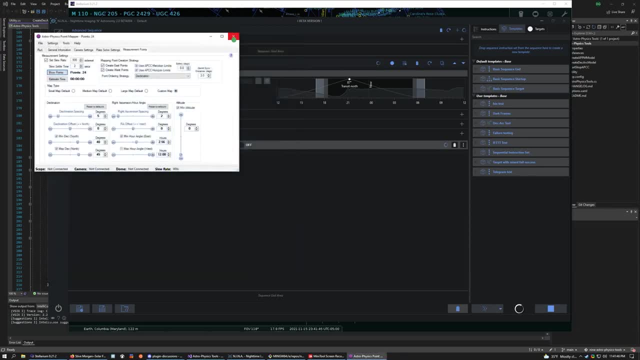 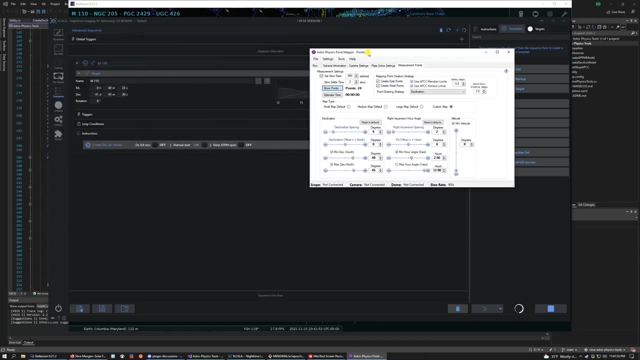 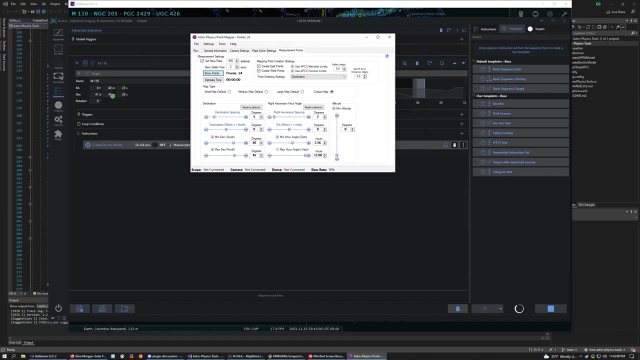 there two arcs, the wide spacing between them, the Andromeda in one tens somewhere there in the middle, and we can verify that by saying: looking at our south limit and our north limit, and then we see that our declination of our target here is at 41 and and three-quarter. 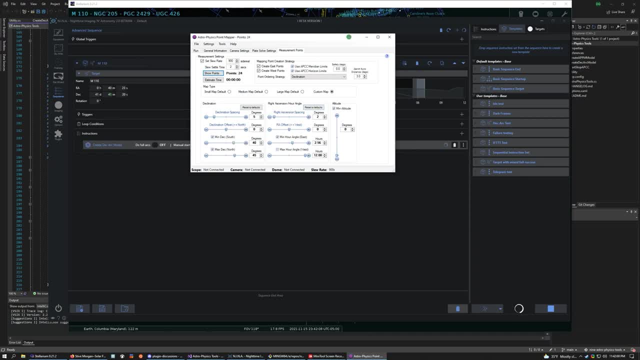 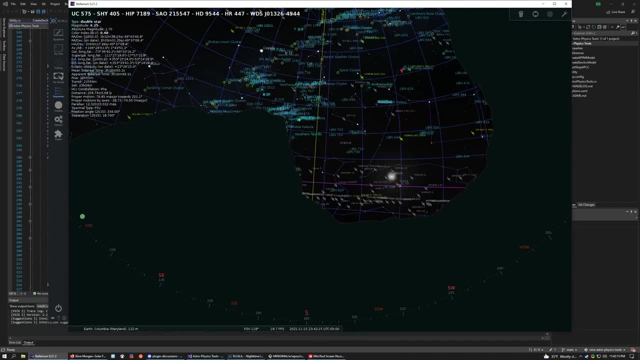 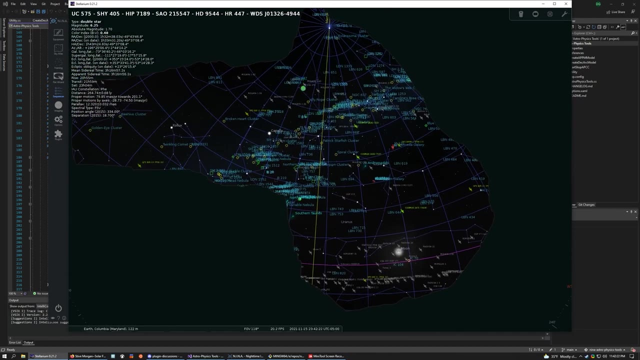 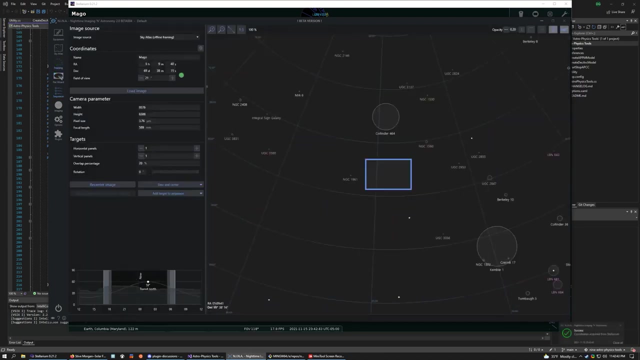 degrees. so right in between, roughly. and let's pick something closer to the pole to show the switch to different RA densities. so we'll pick this. what's this? the Jolly Roger cluster and declination 62. let's pick something closer. yeah, yeah, yeah, Mago, get rid of this. go to framing. so I'll pull it in, create a model, let's go. 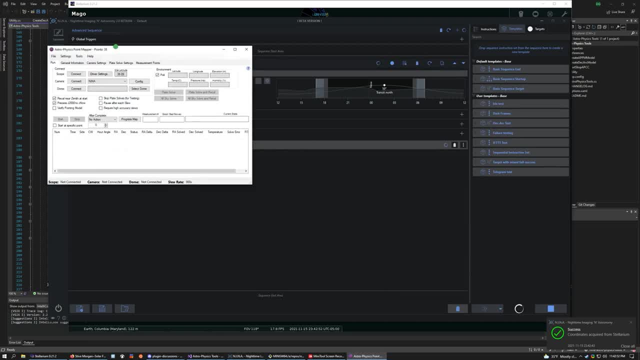 and look at this. this may be like we've moved over here and let's see here, here we go. now we can see this. you of all Louisiana matches. I'm gonna go with this photo. there you go. let's take another look at all these tema. Saint ahí, aliás de jode, CNN. good programming, so I'll pull it in, create a model. let's go and, and let's see here, here, and and let's see if that's what's happening. let's go now. we can seeikel that we need to do a little bit more extreme. traveled American over here now a week ago. but basically, this is a quick discussion. let's�uou manhear hi. we always want to pull a picture here because inside, if you would just come to check out these two tapes, specialty candidates who are now taking the final languages. 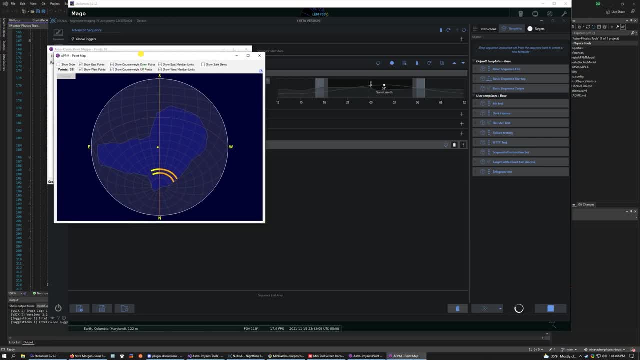 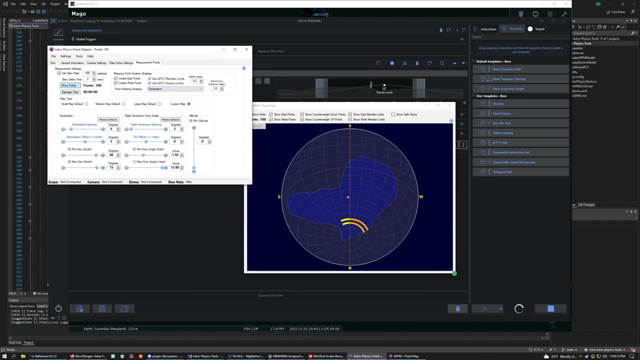 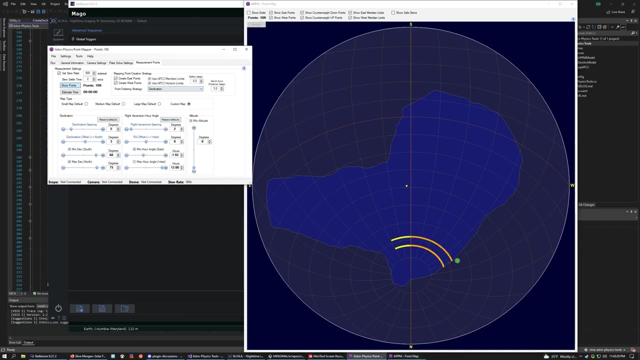 Here we go. now we can see that the model was created with equal RA density per our instructions. If that was created with declination, that's what the model would look like there. So here's the difference: equal RA declination. 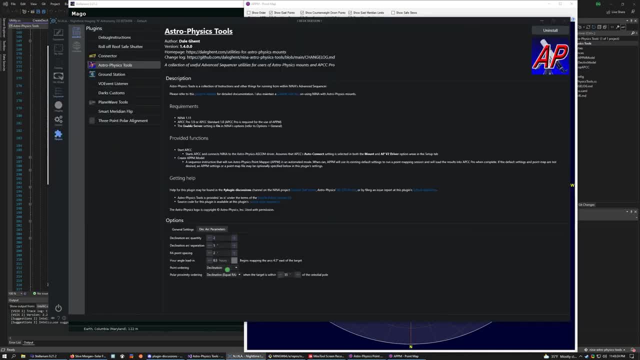 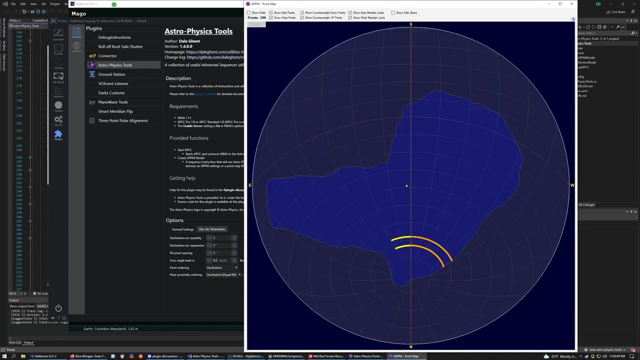 And this is why this polar proximity ordering setting is useful. You aren't stuck to just declination for the entire sky. You can say: within 35 degrees of the pole, I want to do equal RA And you can do that. And this just illustrates that difference between the two.